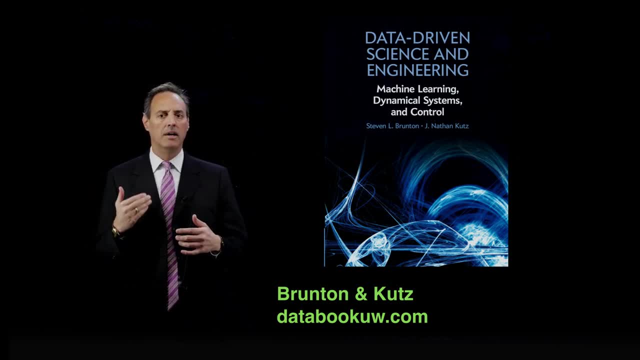 section of the book 5.3, we talked about k-means clustering, which is just a matter of picking cluster centers and associating all the data with one of the two and iterating towards finding a good set of cluster centers, And that's what the k-means algorithm did. So they want to talk. 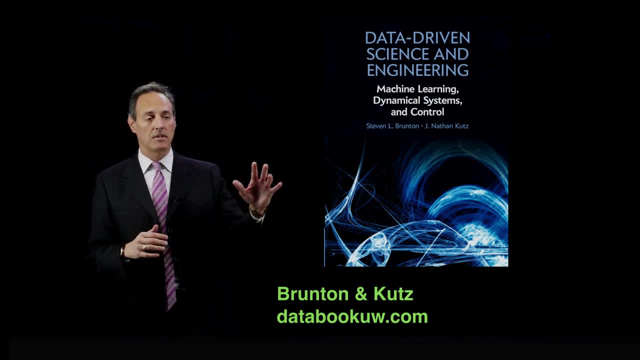 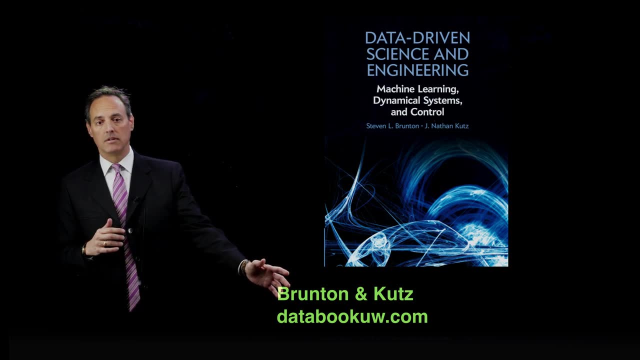 more about what's called hierarchical clustering. This is out of section 5.4 out of the book Data-Driven Science and Engineering, Bruntman-Kutz databookuwcom, You can find many more lectures, lots of MATLAB and Python code. 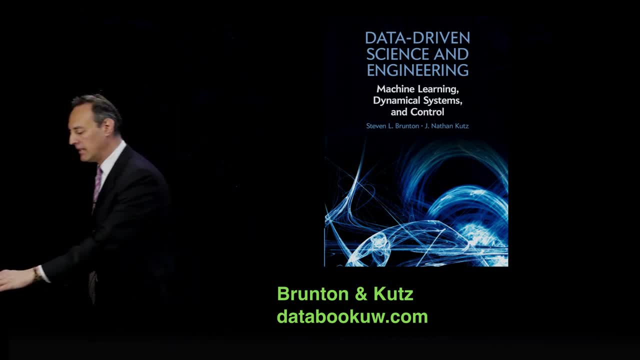 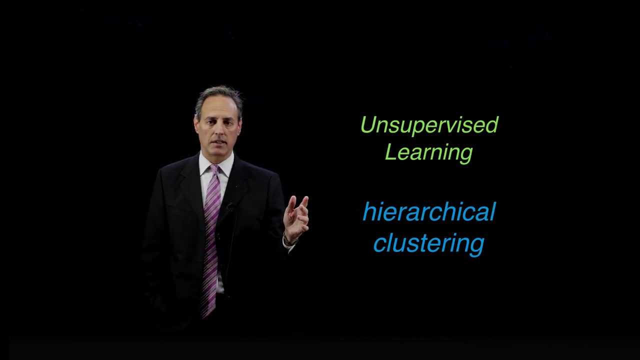 And a lot more video lectures online. So let's talk about this unsupervised learning technique, hierarchical clustering. So it's just like it sounds. We're going to build, start taking the data and start constructing an algorithm, in a hierarchical sense, towards making decisions about. 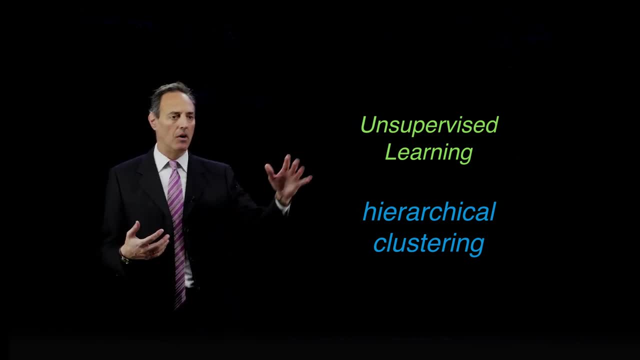 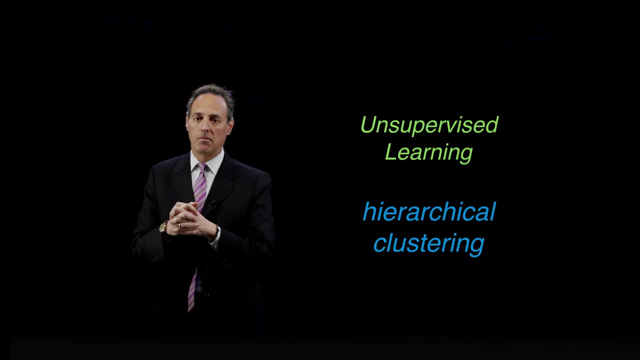 where data sits in a cluster so that we can classify. Now again, it's unsupervised, so there are no labels. I simply give you data And your job is to provide labels for that data in some kind of principled fashion. 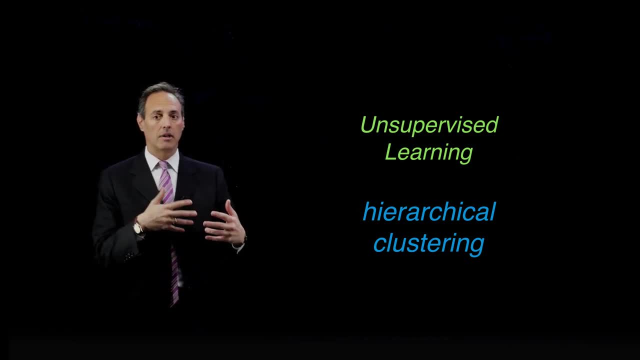 K-means did it one way. Hierarchical clustering is going to do it another way, Just like k-means. there was a decision that had to be made, which is: how many clusters do you want? And in hierarchical clustering- some of that decision process- you can start to see how it. 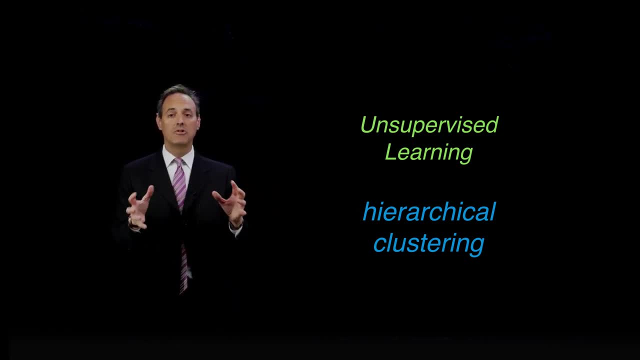 might play out, As I'll show you in a little bit, in what we call building dendrograms, And these dendrograms contain enough information for you to potentially make principled decisions about the number of clusters you want to use in the first place. 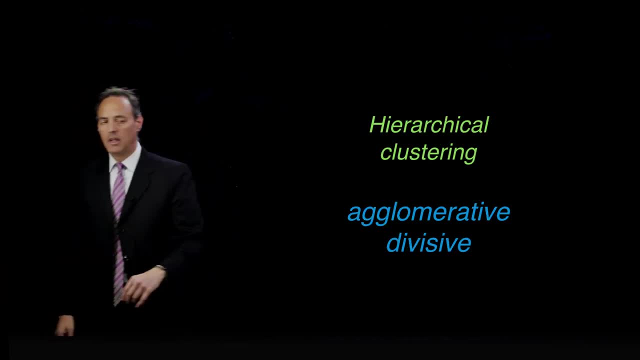 So how does hierarchical clustering work? Well, there's two forms of it: Glomerative- I can't even say the word, You can read it There it is- And divisive. So the difference between these two hierarchical clusterings is the following: 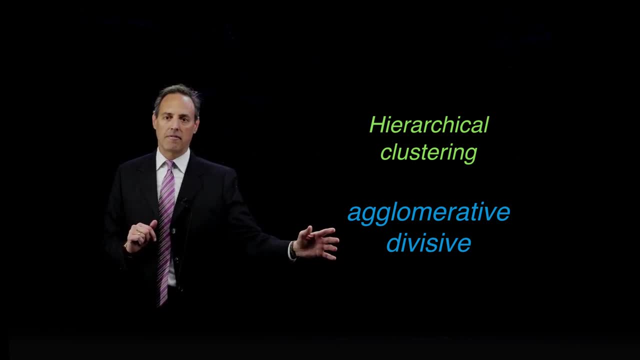 In divisive. let's start there. First, you think about all the data I give you as being one giant cluster, And what you do in the divisive method is you say I'm going to have a principled way to now split it into two clusters, and then three, four, five, In other words, all the way down to each. 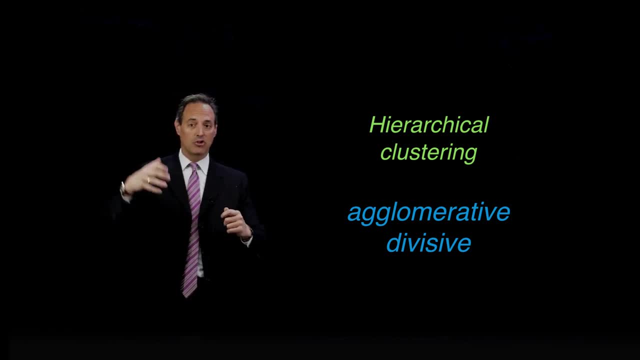 point being an individual cluster. Okay, so you start off with one massive cluster and you find an algorithm that splits it into n distinct clusters where you have n data points. that's divisive. the alternative to this is to instead start off with each point is its own cluster. so you have. 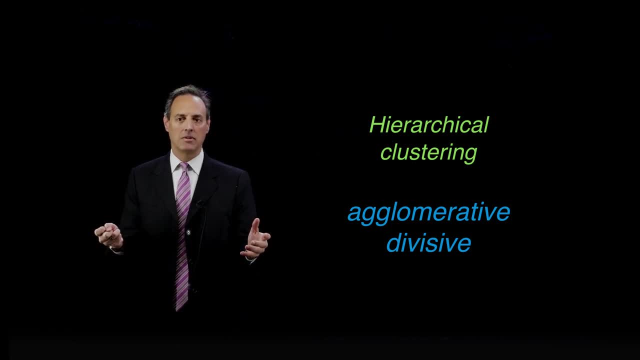 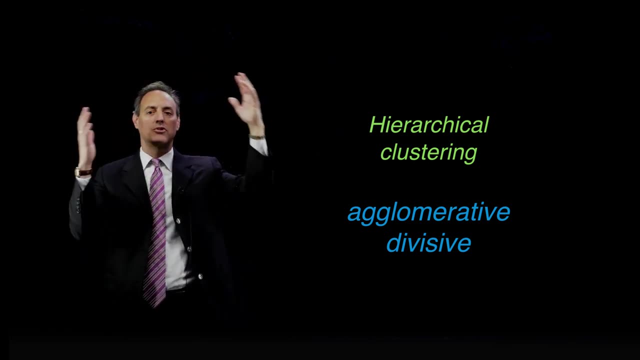 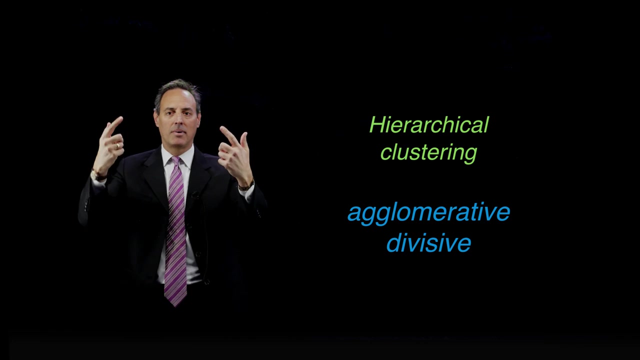 n clusters and then start combining clusters so that you start off with n clusters and you aggregate all the way up to the top to the one super cluster. so in one case you go from bottom up, the other one you go from bottom- sorry, yeah, so bottom up, and the other one you go from up. 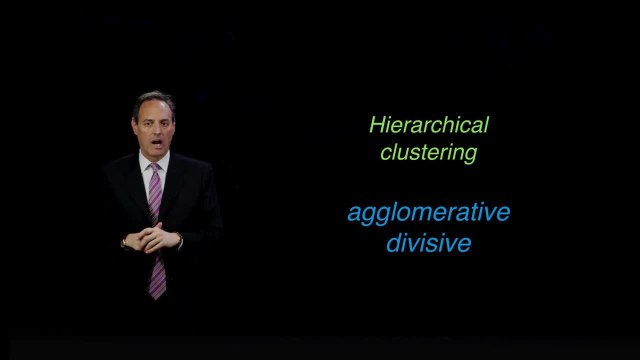 to bottom. okay, so those are the two types of hierarchical clustering that you would have available to you, and we're mostly going to focus in on starting here with starting off with every points of cluster and moving up and aggregating as we go and the way we're going to do this. 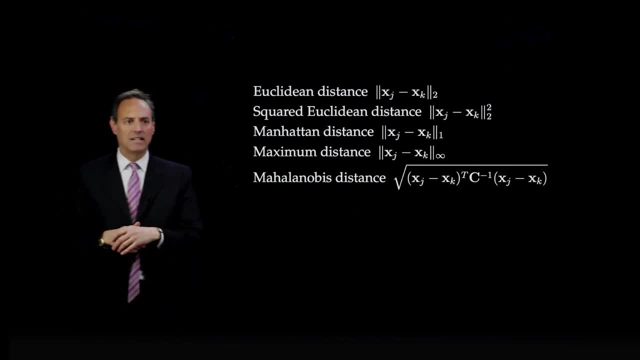 in hierarchical clustering is we're going to have to first define some metrics. what does it mean to be close in space to another data point? so this is a really important issue, because how you measure this determines a lot about how the clustering is going to happen, and I'm what I'm giving you. 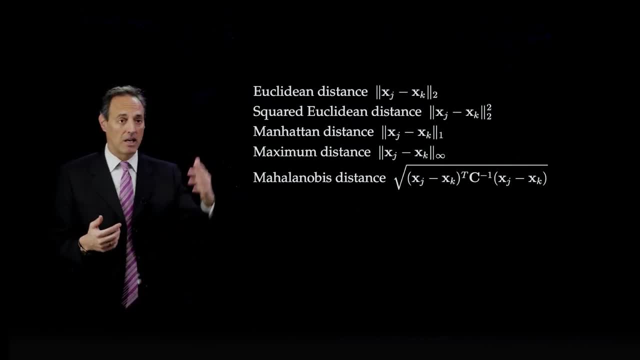 here is a set of metrics. you can always just use your standard. look Euclidean distance. right, it's an L2 metric between two vectors right X, J minus X of K norm squared. or actually that's the Euclidean, The square. Euclidean is with the square. 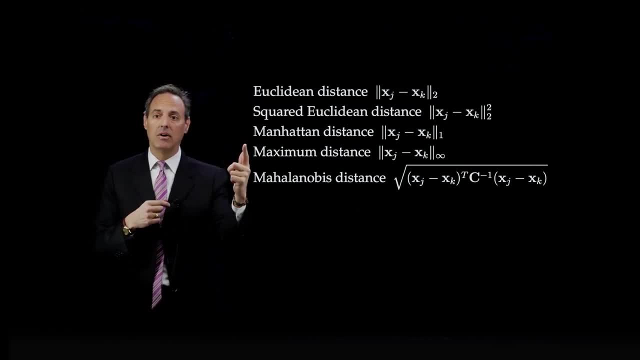 There's a Manhattan distance. This is the L1 norm, And we already talked about in chapter four the differences about regularization using different norms, whether L2 or L1, because those metrics really matter And here again you see them showing up. 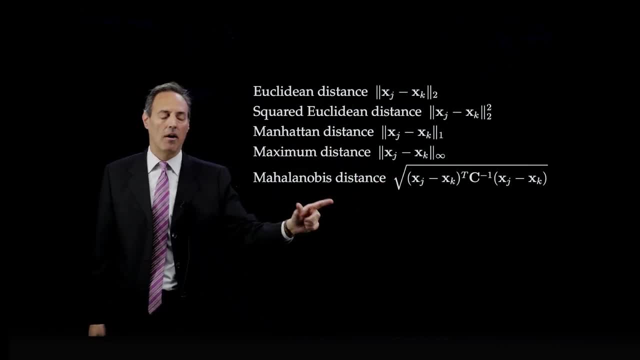 here You have two norms. You have one norm, infinity norms, And then you also have this thing called the Mahalanobis distance. So these are different metrics you can use to measure how far one data point is away from another. Your choice of metric will give you, can give you. 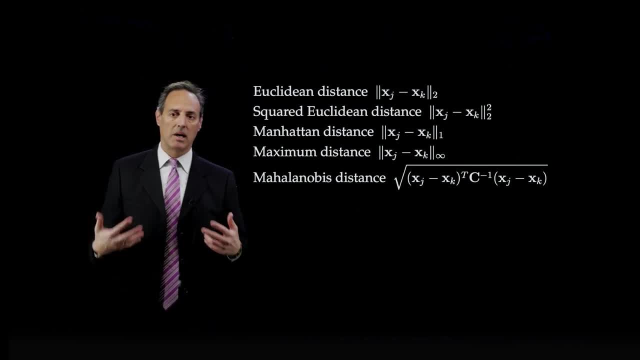 significantly different results, So just keep that in mind. In fact, the choice of metrics might be exactly what you need to give you results that make sense and are meaningful. Some metrics may give you Just nothing that you can really make good decisions with about your data. 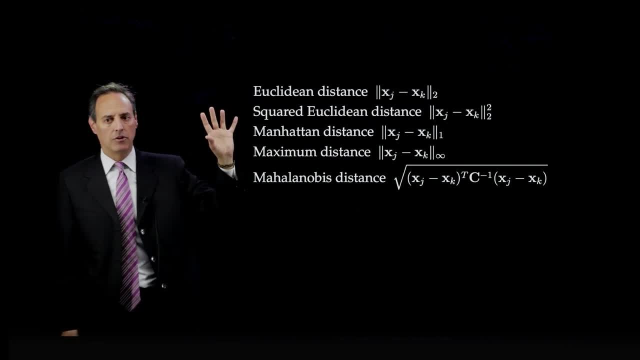 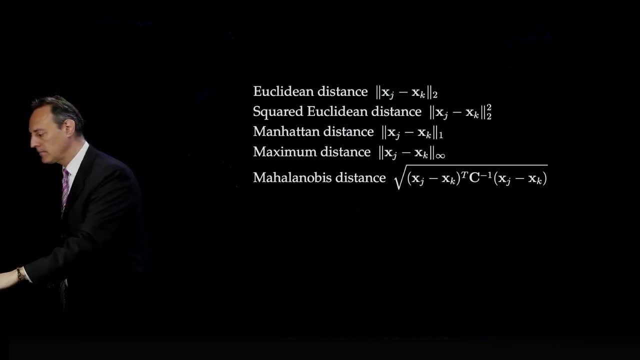 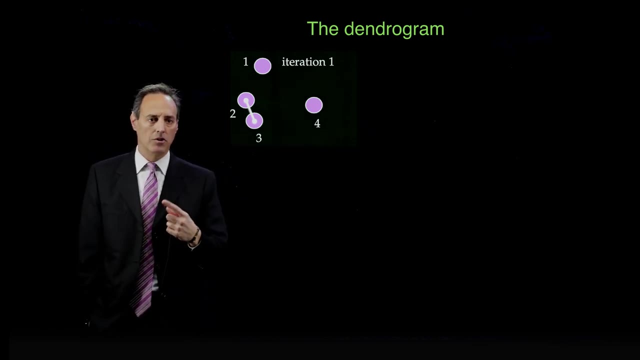 So I'll just leave that out there, And the hope is that you have some intuition about your data, about what metric you should use as the best for that data set. So let's talk about what's called the dendrogram, And this is going to be the hierarchical clustering we want to do. 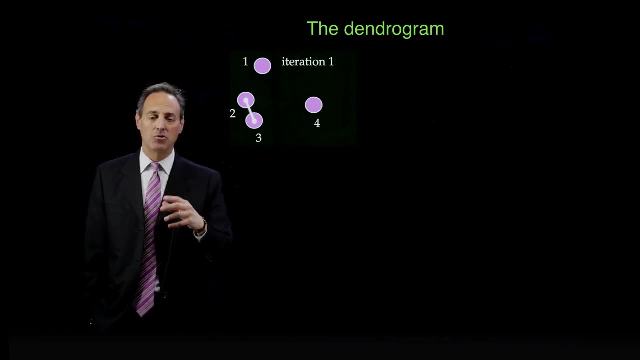 And I want to show this algorithm in sort of in its usage And very much like k-means. you can just simply execute this algorithm. There's not much thought into it, There's no optimization, It's just simply. you know, in k-means it was an iterative algorithm. 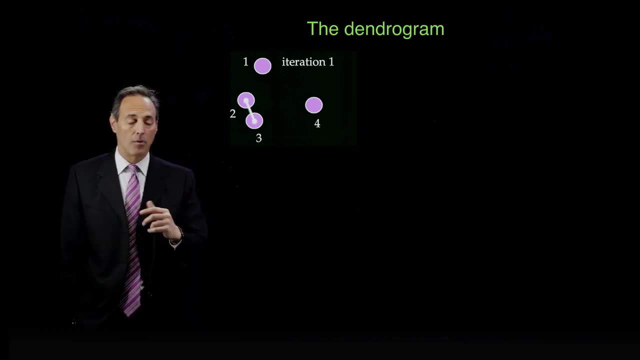 And same thing here. You're just going to walk through this algorithm And you're going to start off with all of your data points and clusters and walk it all the way up to there's one giant cluster. Okay, All right. So here's how this is going to work. 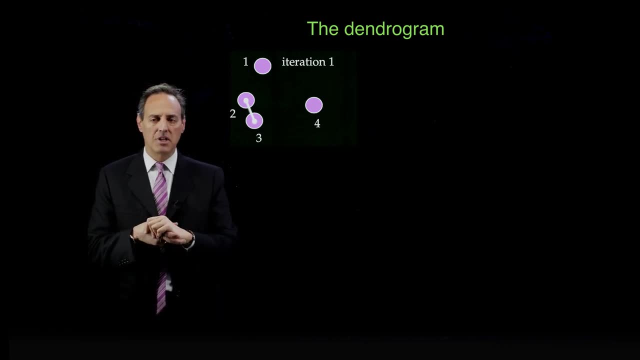 Those magenta balls are your data, And what the dendrogram is going to do in the first iteration is say, out of all those balls which two are closest Okay. So the costly part about building this dendrogram is for any point. 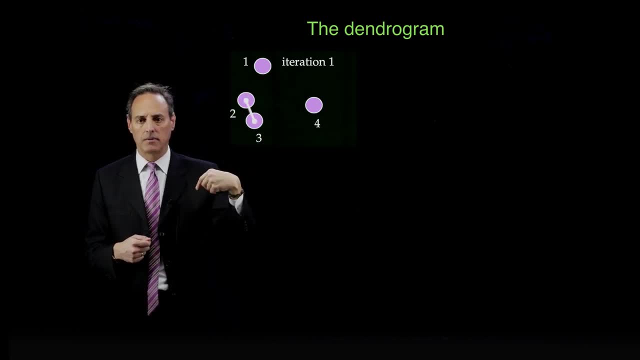 I've got to compute my distance to all other points. Okay, So that can be expensive, especially for very high-dimensional data. There are faster algorithms for doing this, where you only look in a neighborhood, so you don't look at the distance to all points. 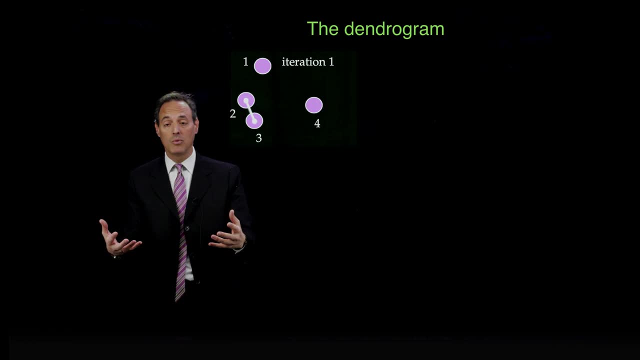 You just look at those around you, But first you have to figure out who's around you to begin with. But once you have some information you can actually cut the computation down. So in this case, here points two and three are closest together. 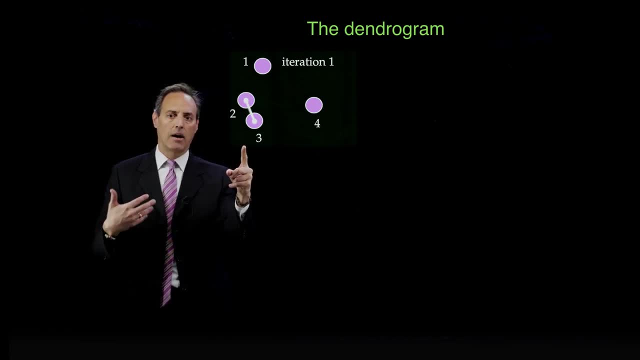 So now, what the dendrogram is going to do, or what this hierarchical clustering is going to do, is to basically merge these points into a single data point, And the single data point will be at the midpoint between them. So this is the idea. 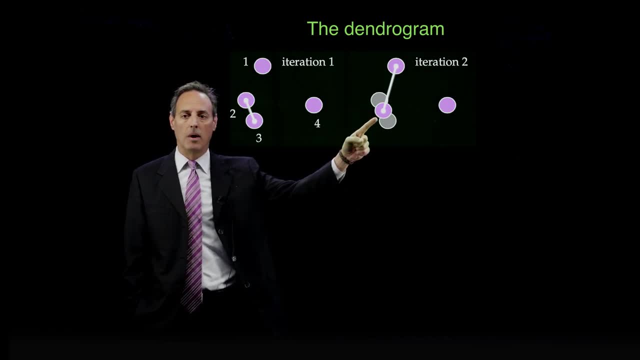 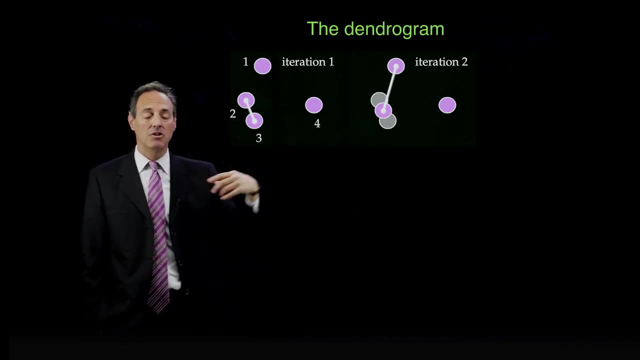 So now, I started off with those two points. I've now merged them. I've merged them into one point. I'll now have three data points, not four, Three magenta balls, And I do the same thing as before, which is I say: 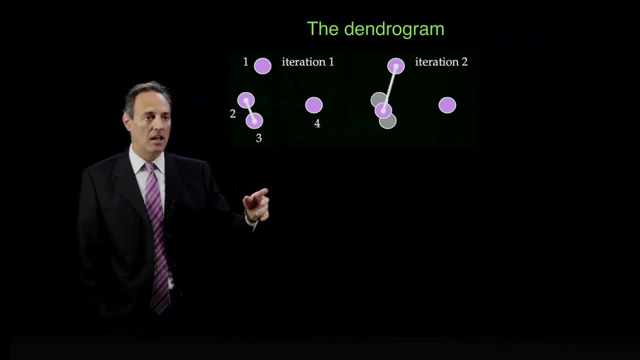 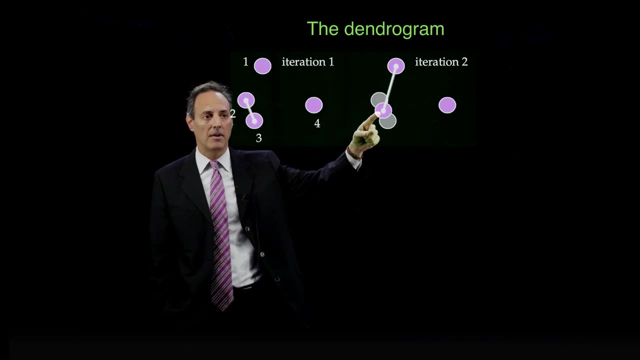 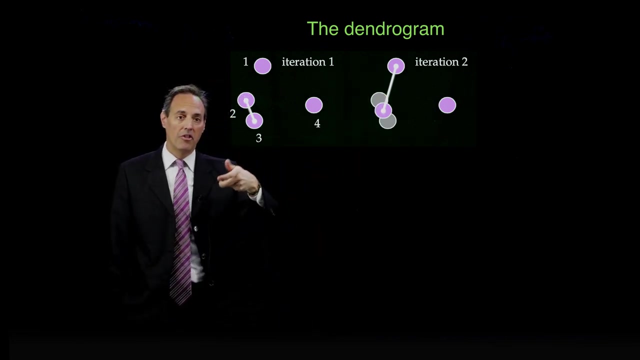 now, what is the distance between all the data? And now, in the second iteration, you can see that this point one to this new joint point two, three together is in fact the closest distance. So what I'm going to do is join those two together. 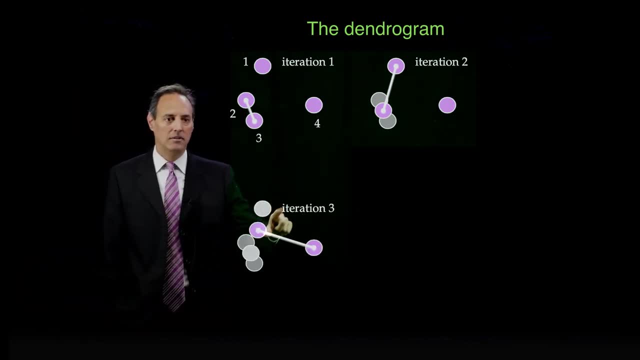 So now on the second iteration, these two here get joined together into that ball right there. So now I have two data points And of course there's only one distance. I have to compute between them, And now I just basically take the midpoint and that's now my new data point. 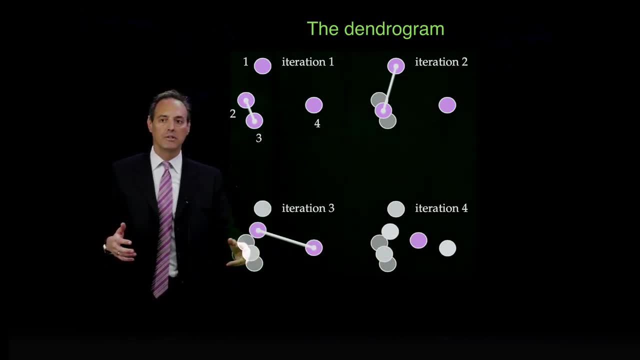 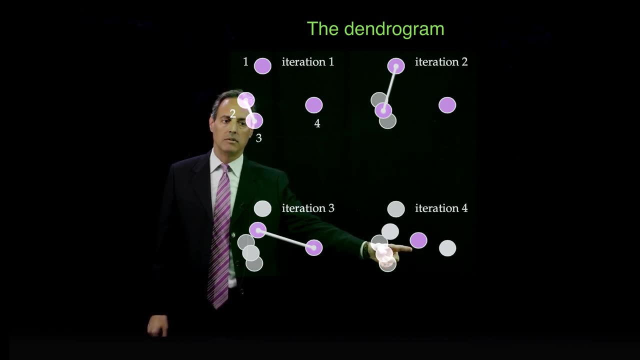 There it is. So notice what I did. In four iterations I started with four data points and I ended up with one data point at the end of four iterations. So I aggregated all the way up from four to over four iterations to one. 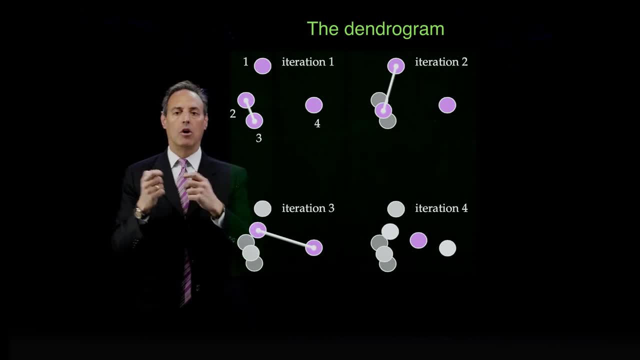 The cost of it was I had to compute distances at every round between all the points so that I can make a decision about who was closest. So, again, your distance metric matters, And what I've just shown you here is something like your standard, you know, L2 metric distance. 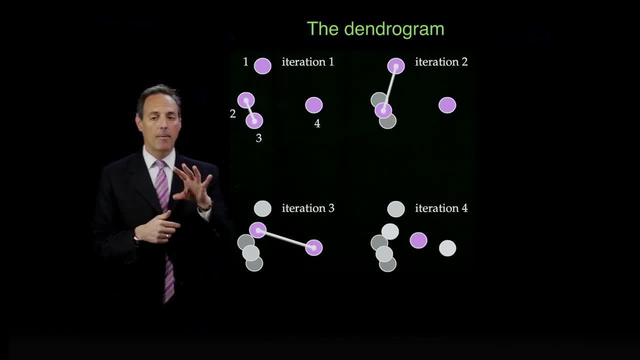 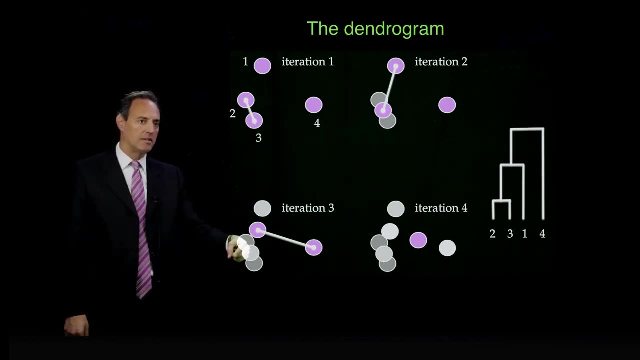 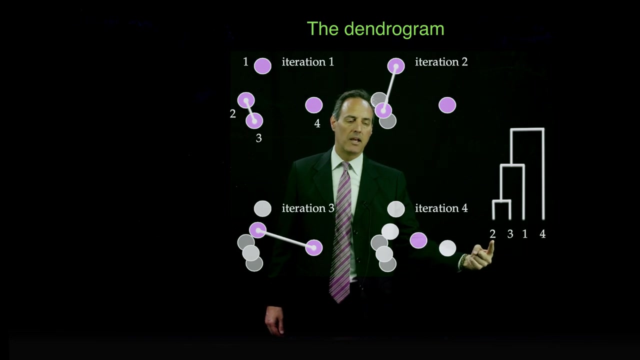 between points. Okay, but you could use others. Now, how to represent this in a dendrogram is. I'm going to show you this picture. This is the dendrogram associated with this process. What I have here on the x-axis is the label for the data point: Data point 2, 3, 1, 4.. 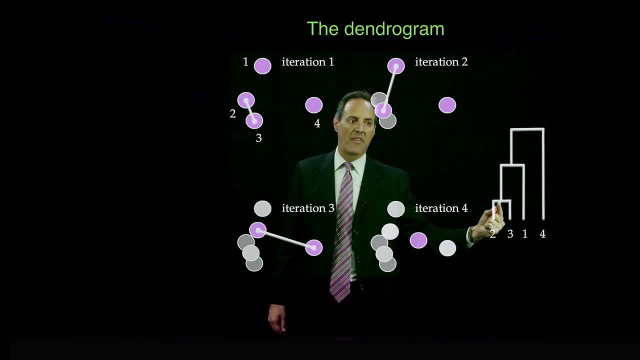 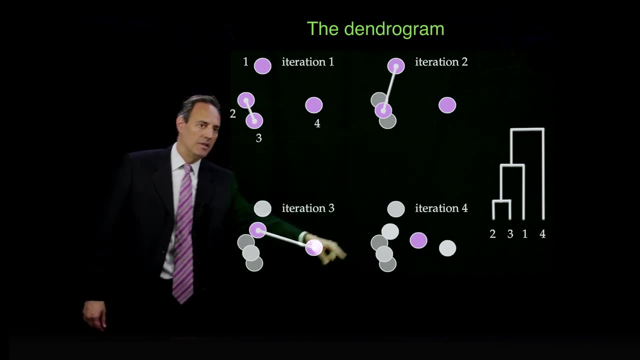 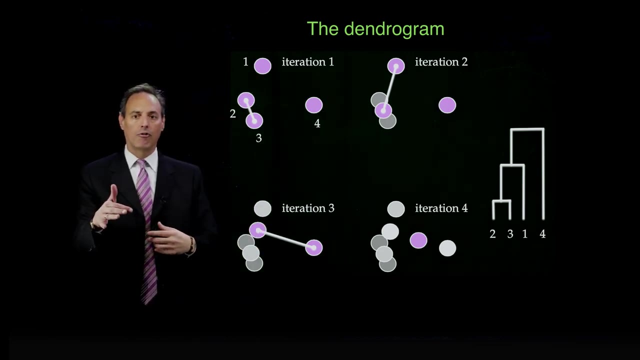 What I first did is I merged 2 and 3.. Now that merged point merged with 1.. That then merged with 4.. And that's just shown here in this iteration structure. So this is called a dendrogram. It shows you in a graphical form the merging process that happens in this. 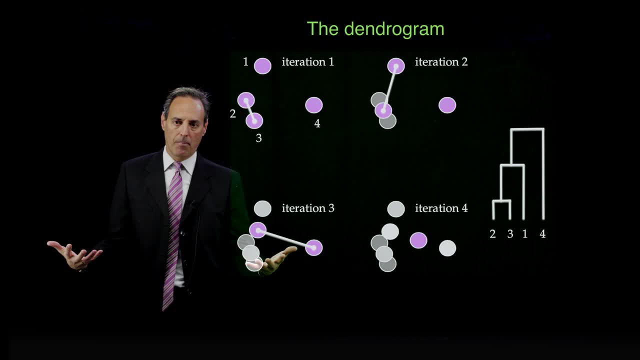 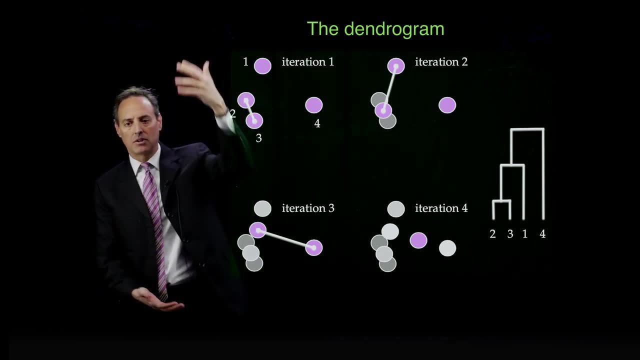 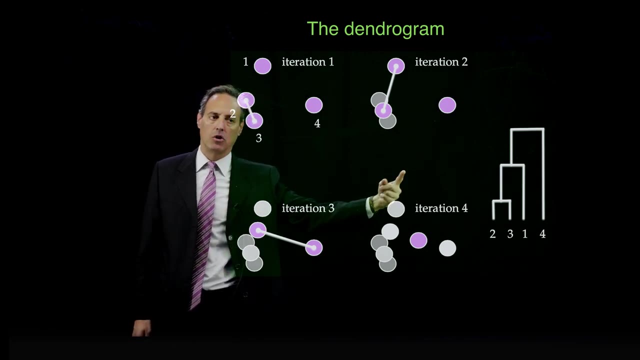 hierarchical clustering Going from n data points to one cluster. So you know everybody is their own cluster- to being one cluster. How you do the merging is just simply based upon distance, but you can represent it. You can represent that in a picture like this, which is called a dendrogram, And often 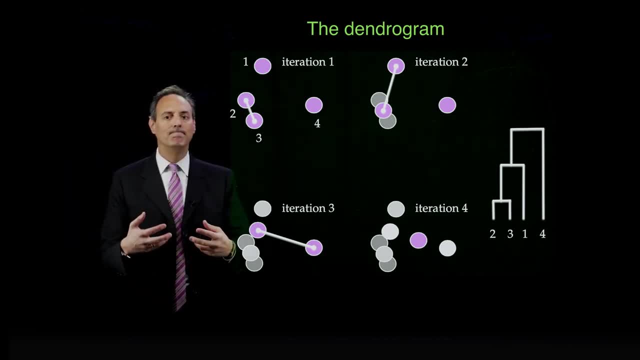 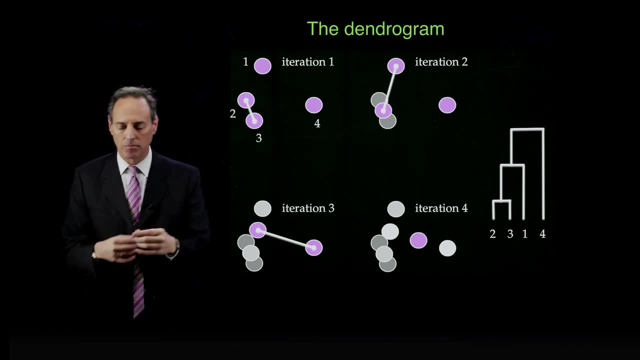 times, dendrograms are highly interpretable. That's the important thing: what a dendrogram is trying to show you. In fact, I'm going to give you an example when we go some code in a minute here, of what this looks like. So let's go to some code And in fact I'm 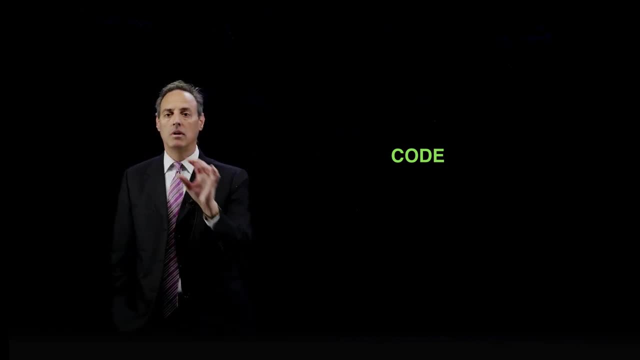 going to do the same example I did in the k-means, which is I'm going to give you two distributions of data. One is going to be a stretch ellipse, Another is going to be a networklad in our graph, And one is going to be a cluster and another is going to be 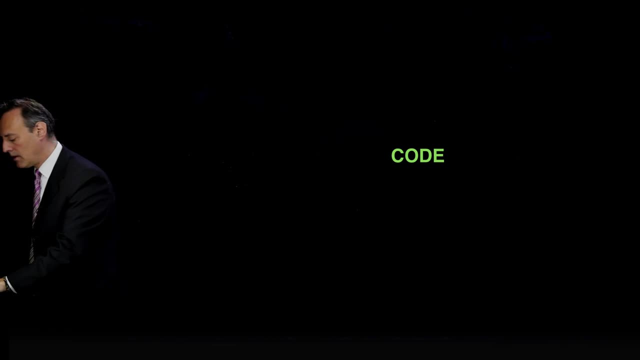 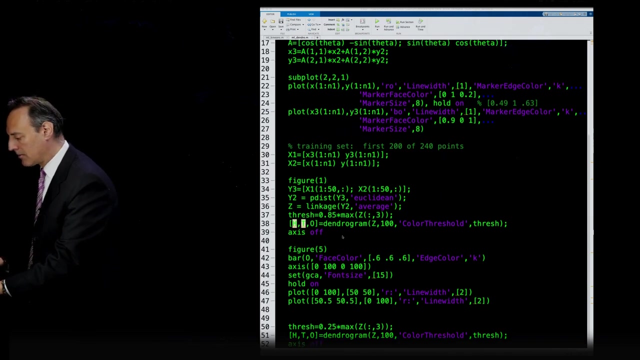 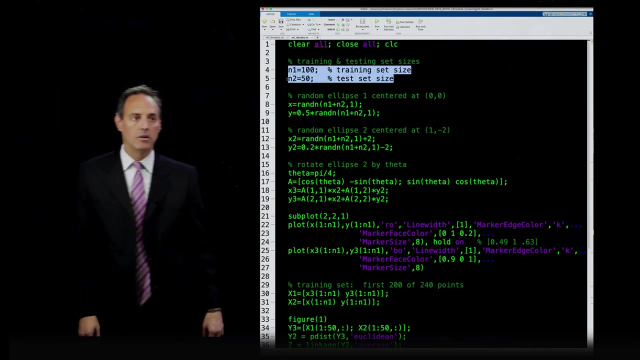 just some random Gaussian distributed And then we're going to do basically hierarchical clustering on those. All right, so let's come here, put this down. So what I want to do here is I'm going to walk through this dataset here. So, first of all, very much like what I did in k-means. 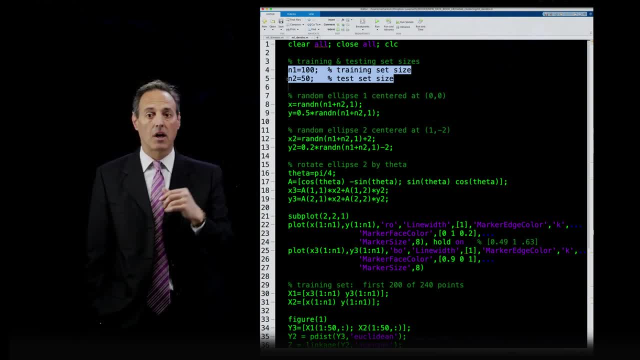 what I'm going to do is take some training data and test dataset cause. once I have the hierarchical clustering and where the cutoffs are between the hierarchies, I can use this on new data. for instance, I'm going to generate two data sets. 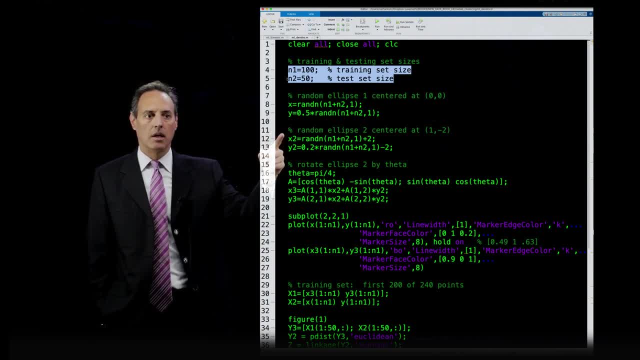 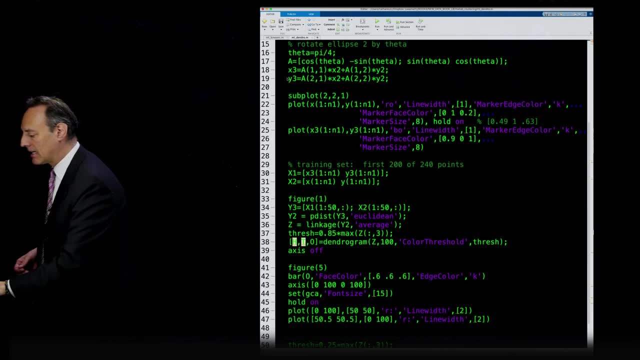 First, I'm going to generate one distribution, a second distribution. I'm going to rotate the second distribution, so it's going to look like a little Gaussian stretched, and that's going to be my data that I'm going to use here. 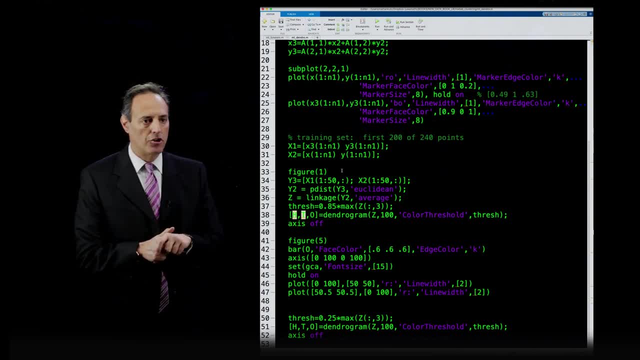 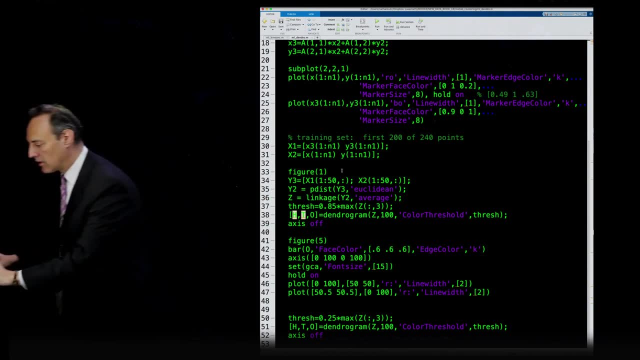 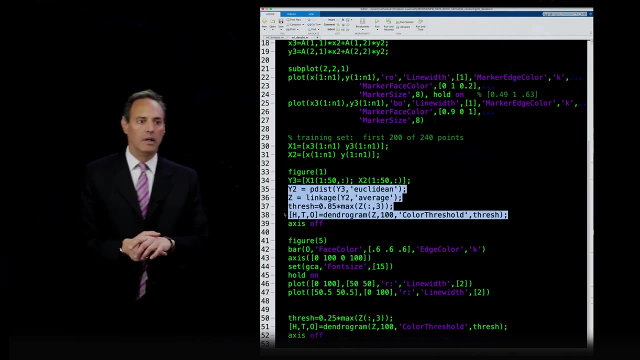 Now, once I have that data, what I'm going to start to do is start to create the dendrogram structure itself, and that's done here in the code. So let me just show you This is the code- and it's as simple as that- for generating the dendrogram. 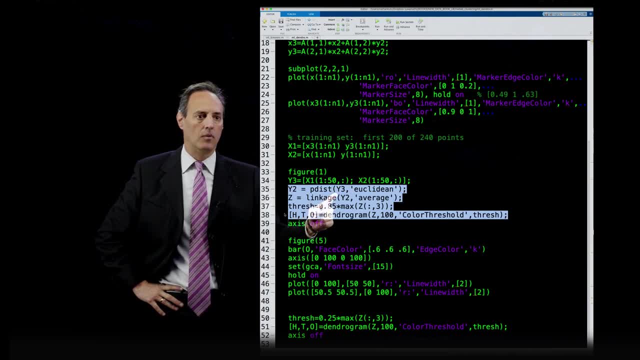 So first of all, you take your data. Here it is Y3.. So what I've done here is taken some of this data. In fact, I've taken 50 data points, Y3,. take this: PDIS is probability distribution Euclidean. 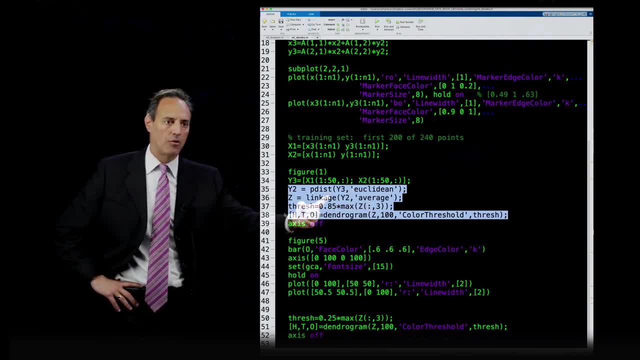 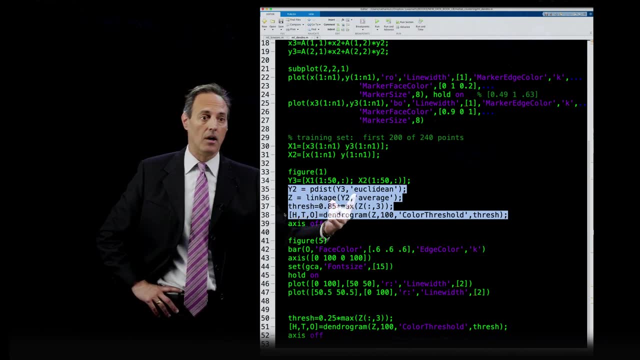 So what I'm going to do is: this is my distance metric that I'm using, and, of course, you can change out these distance metrics as you please. You can make them a Halanovas distance. You can do other kind of distances you want. 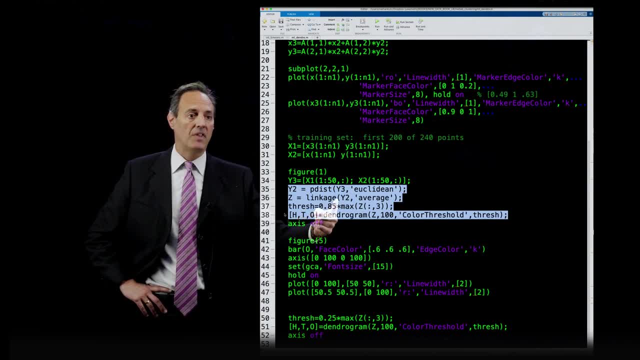 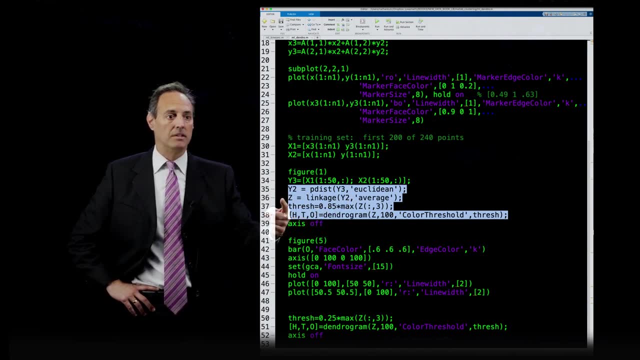 This is Y2.. Use this linkage command with that new data. Again, you can put in some modifiers. here I'm using the average to create Z and then I can define a threshold. Now the threshold is going to tell me how many distinct clusters. 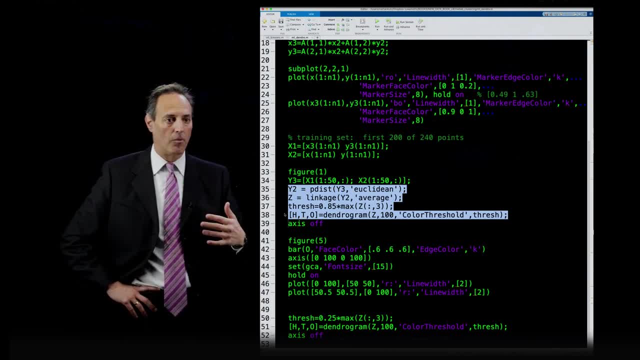 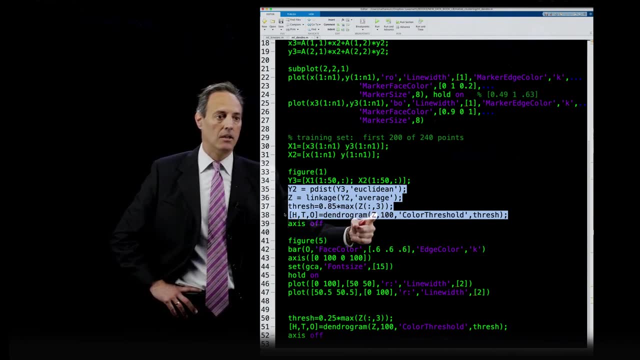 I want at a given threshold level. I'm going to show you the pictures here in a minute and then you just simply take dendrogram, take this linkage data: Z color threshold thresh. So I'm going to basically show you the thresholds in color. 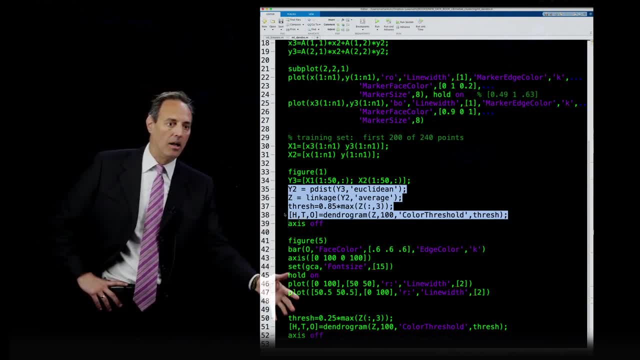 and I'm going to get back the metrics H and T and plot what those look like here on a dendrogram. So, in fact, actually, this will plot the dendrogram for you right here. Okay, I can also take a different metric. 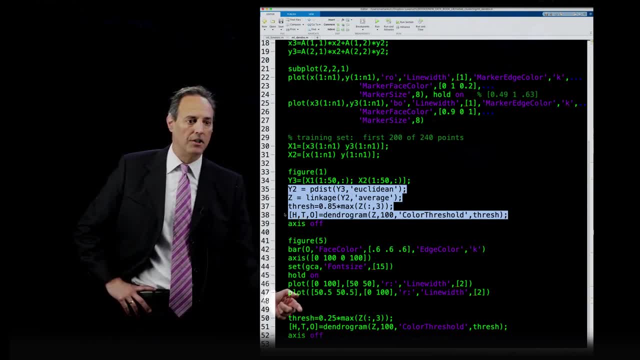 I can take a different threshold, which is what I've done down here. My threshold down here is now at 0.25 versus 0.85, and I'll show you what the difference of these look like in practice. So if you run this, you'll create your dendrogram. 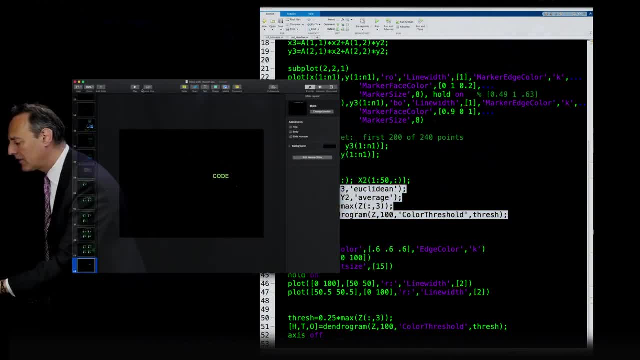 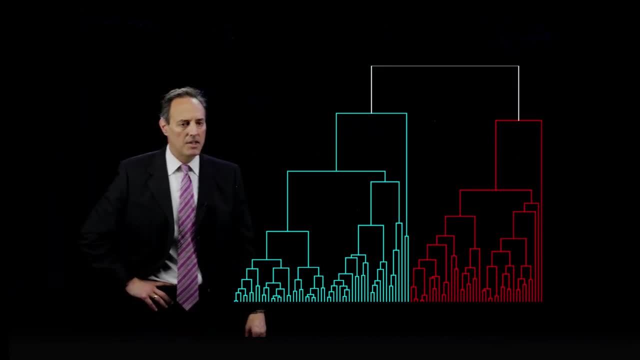 Let me just show you the results here. I think they show up better here in the PowerPoint slides, so I'm going to do it here. Here's your first dendrogram. What it did is took those distributions and it basically constructed this following dendrogram: 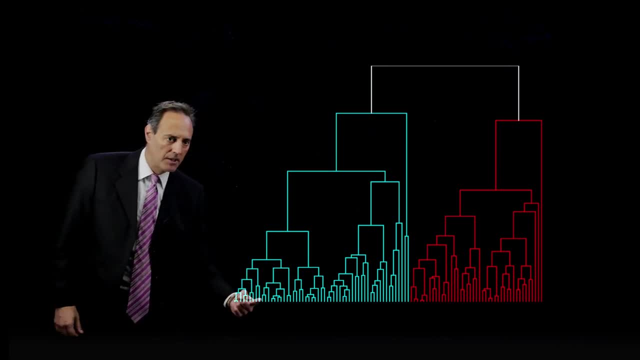 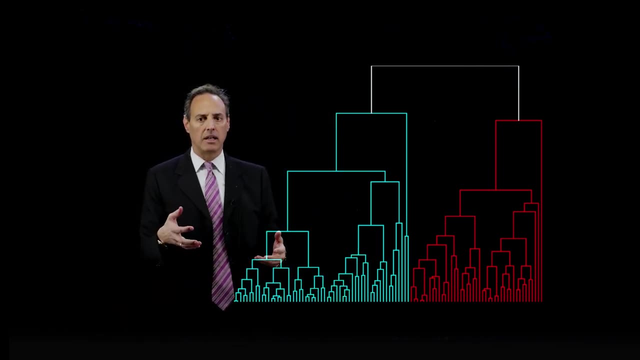 This is a dendrogram through hierarchical clustering. Again, you can see the joining process that happens from this low level. This is all the data and how it gets clustered to its neighboring data. Again, it goes all by distance, whatever distance metric you pick. 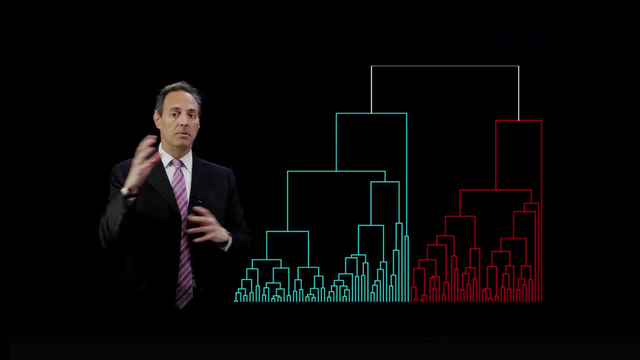 which was Euclidean. here It just simply says, out of all the possibilities of pairs of points, who is closest to each other? That's the first split. And then you see these bars across here. tell you when these joinings happen. What's interesting about the structure of the dendrogram is you can see by setting. 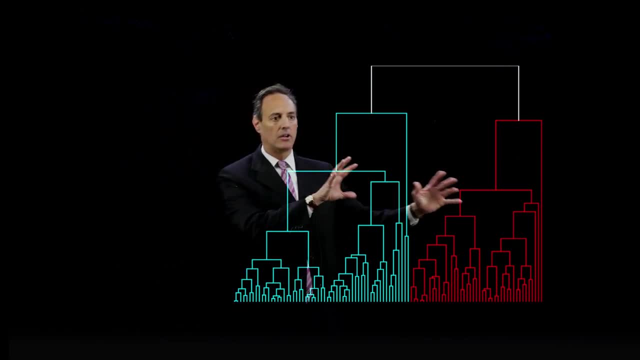 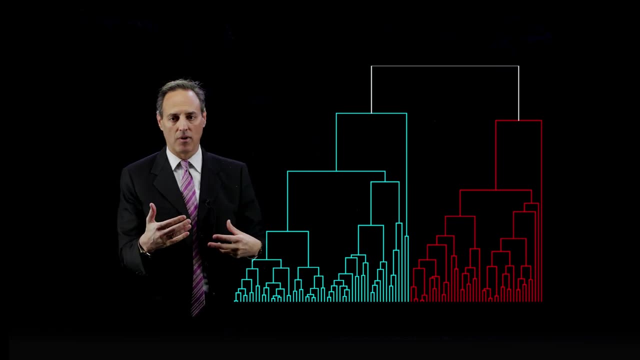 that threshold. it says: look, by setting a threshold, I think you have two clusters, a red and a blue cluster. So it's starting to pick out how many clusters it thinks you have based upon the thresholding command. okay, So that's what it does here and it's a very nice representation of the data. 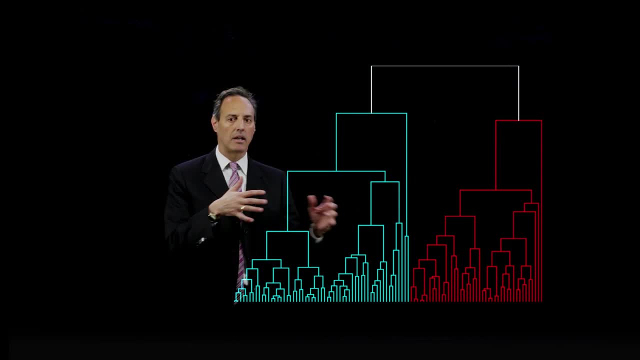 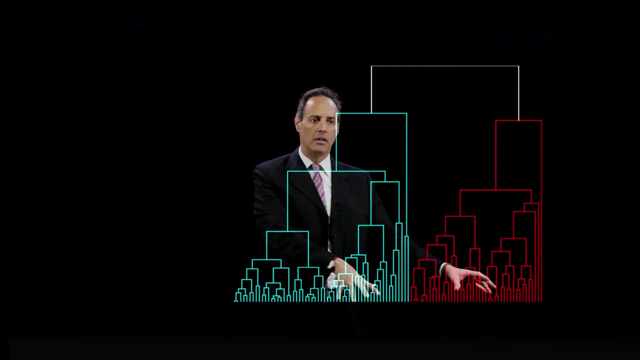 So right away, from a visual inspection point of view, not only did you see the aggregation process, but you also saw that there's sort of these two major branches where the data comes down in this hierarchy. So that tends to be fairly informative for people to start doing diagnostics on the data. 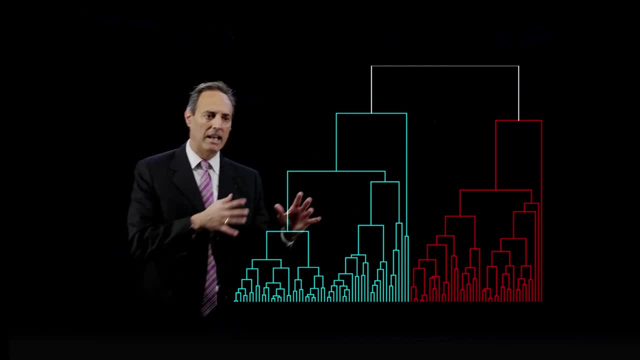 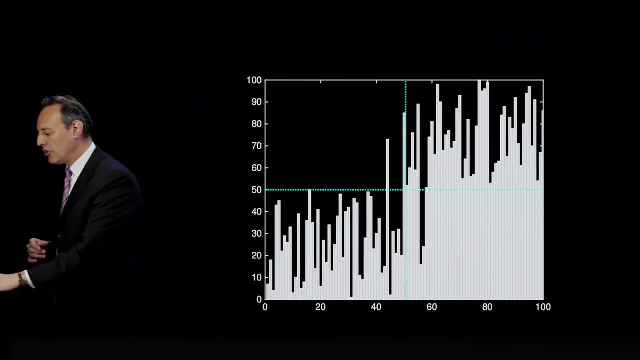 Again, completely unsupervised, so you know nothing about this data. and now this is telling you something about your data And now you can dig down on that. I could also go back to my original data, and here this plot is important- to see how well I did. 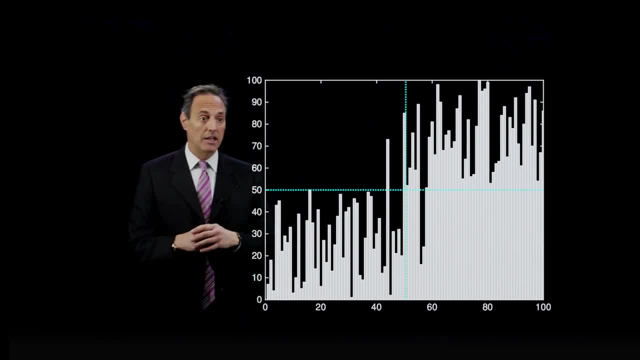 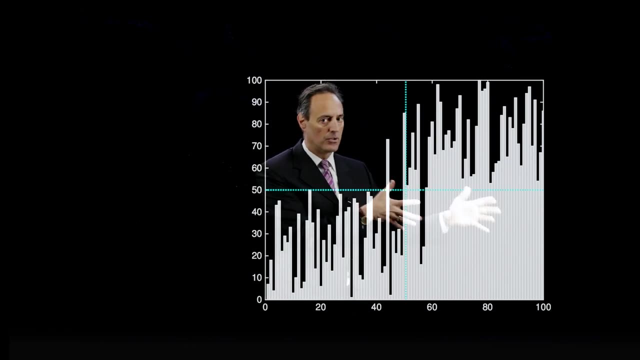 So I had two clusters of data from two distributions And so I drew this blue line in the middle and this blue line here. All of the points- the first 50 points are supposed to be from one PDF that I generated the data. the second are from a second distribution of the data. 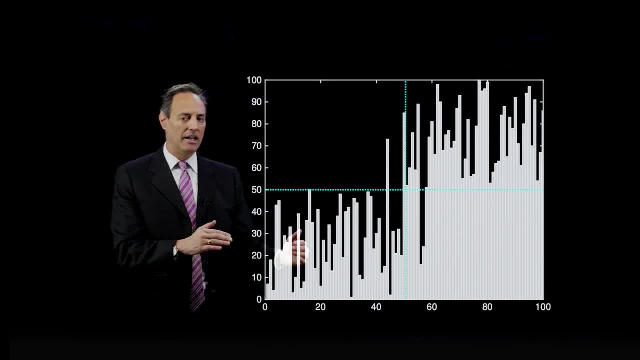 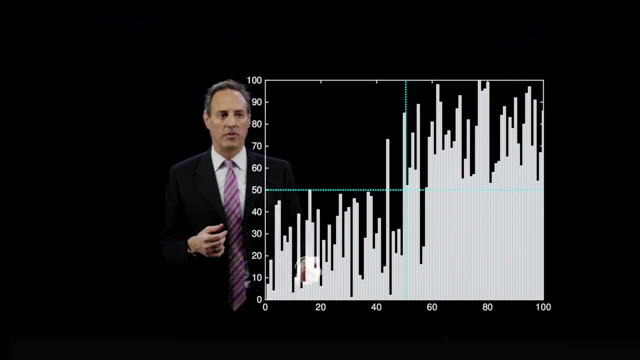 So one way to think about it is: everybody below this line should belong to the first cluster. that's the truth. Everybody on the other side should belong to the upper cluster. that's the truth. And so you see, it actually doesn't do so bad. 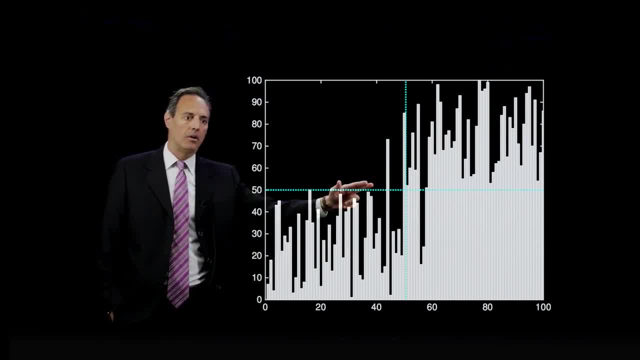 In fact, if you look, if you look at the upper cluster, that's the truth And so you see it actually doesn't do so bad. In fact, if you look here, there's only a data point that really goes above this line. 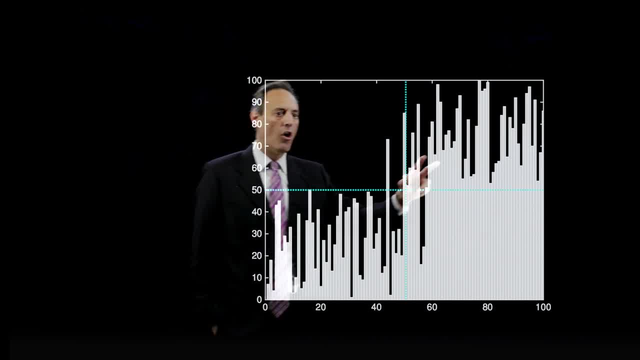 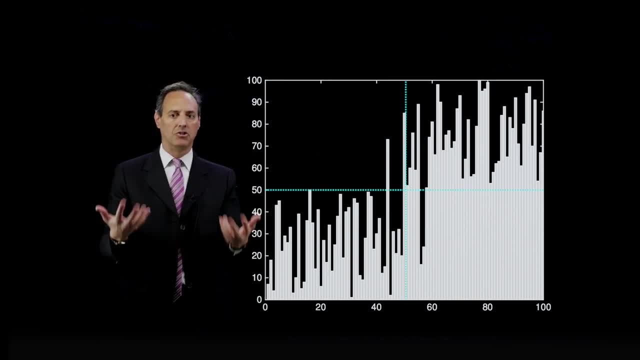 It's actually, I think it's- two data points in one. There's some that are close over here. some gets mislabeled the other way. So I have these two PDFs, two probability distribution. This was the artificial data I generated. 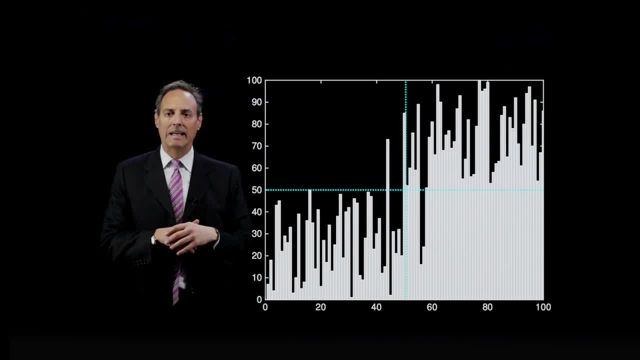 When I do the clustering on this data, you can see it actually gets most of the labels correctly. So in a completely unsupervised way, I didn't give it any information and it backed out information. I gave it all the information about the data I put in. 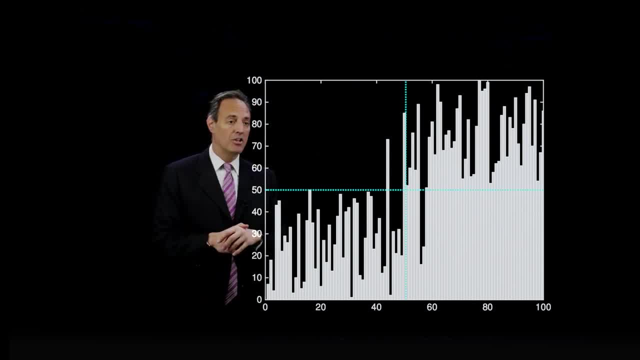 which is two PDFs with two probability distributions. So this is kind of encouraging in the sense that the dendrogram is keying in on major pieces of the data and it's all based upon distance metric, So that's an encouraging sign. In fact it does quite a bit better than k-means. 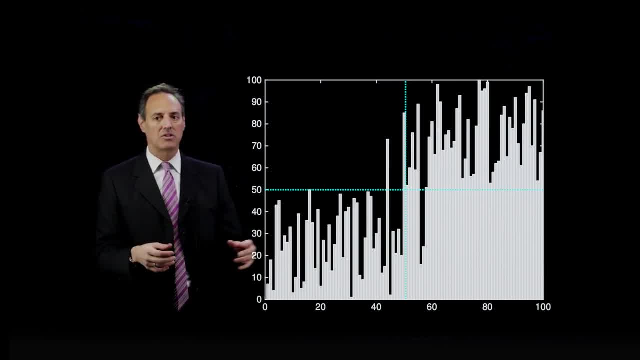 Cuz- k-means remember- is trying to do centroid clustering, where this just says whoever I'm next to is gonna be who I'm gonna basically partner with In a cluster. So you're more likely to get this to actually work out well in many instances. 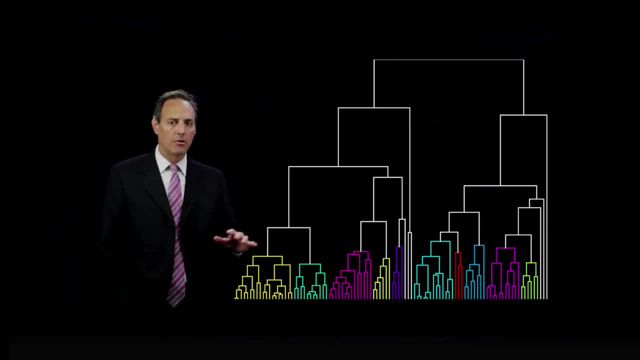 You can also play with that threshold and the thresholding will allow you to split it into more structure in the data. So, for instance, by playing around with that threshold. here's a new picture of this, where every single different color here is a different cluster.